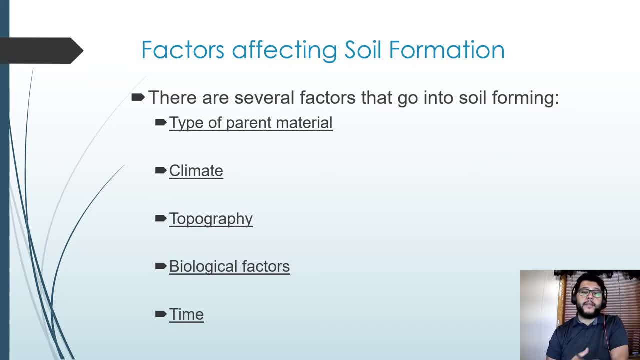 that rock formed. So if it's a climate that has very dry weather with not a lot of water, that's going to play a big role in how that soil forms. If there's a lot of mountains or if it's flatland, that's going to play a big role on what layers form first and what layers form most distinctly. And 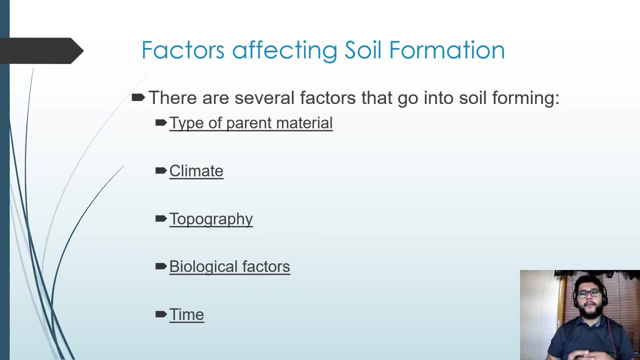 then you're going to have the biological factors, which are things like bushes and roots and trees and grass. right, Think about a tree with a taproot. Taproot is going to be that kind where the root falls straight down and then spreads out. That may play a role into how that soil forms and 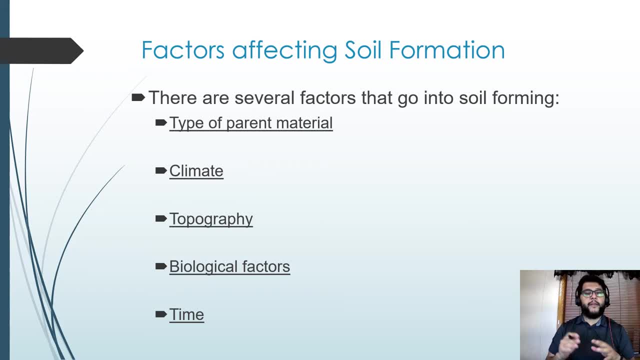 breaks down, Or if it's not a taproot, if it spreads out kind of like grass, as kind of a mesh netting, that might be more helpful in keeping that soil from erosion and things like that. right, And of course, the biggest factor with all these is going to be time, right, How? 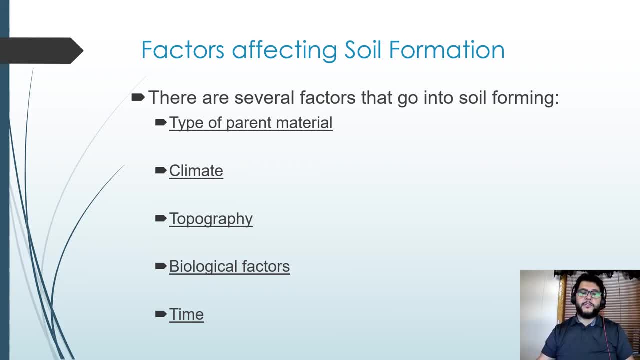 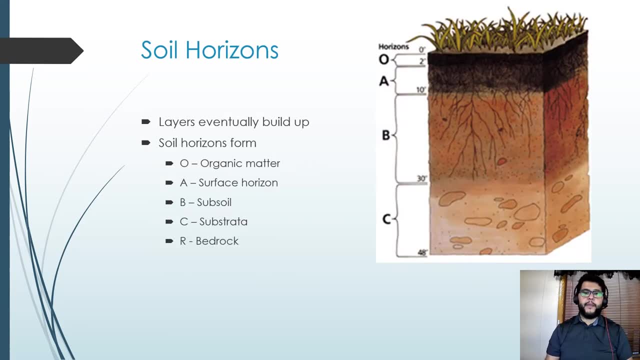 long has that soil been there? Is it going to be able to form into the clear layers that we're going to be talking about shortly? And, as you can see here, here are those layers. So you have the different soil horizons And I hate to say to memorize things, but this is definitely one you 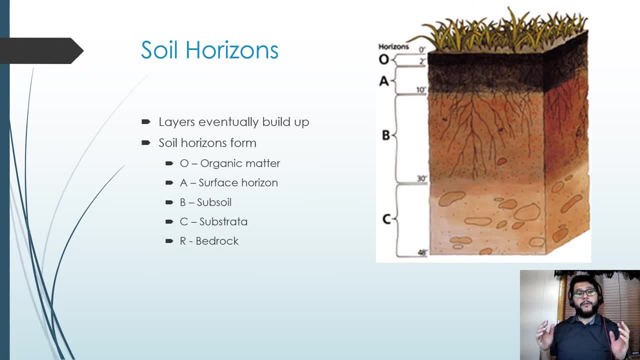 have to memorize and know for the AP exam. And so you know, the top layer is going to be that O layer, That's the organic matter. okay, Then the A layer is going to be right below that. That's going to be the surface horizon, That's going to be the soil. that's going to be the soil, that's. 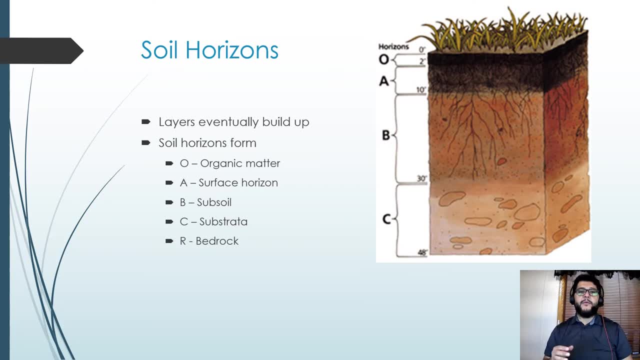 going to be that top layer that doesn't have as much organic. The B horizon is going to be your subsoil. That's where a lot of the roots will go down into. Then you've got the substrata, which looks a little bit like the parent material, And then I would add even another layer below that C. 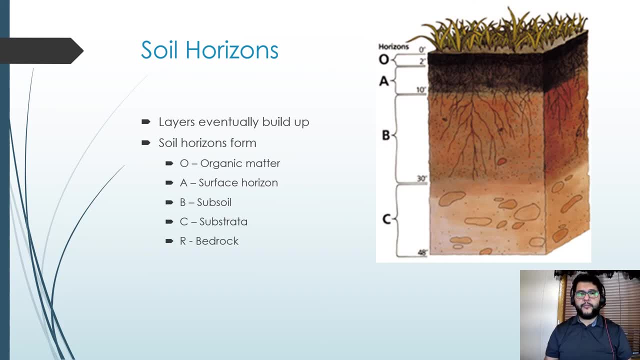 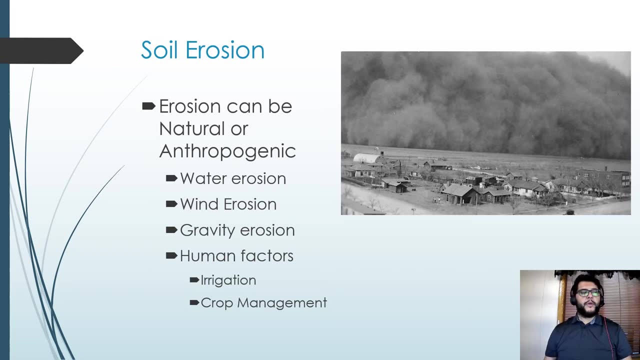 one that would be the bedrock, That's the parent material itself. And then here you have soil erosion. So erosion can be natural or it can be anthropogenic. What that means is that soil erosion can happen on its own through rains or winds. And then we have anthropogenic, which means 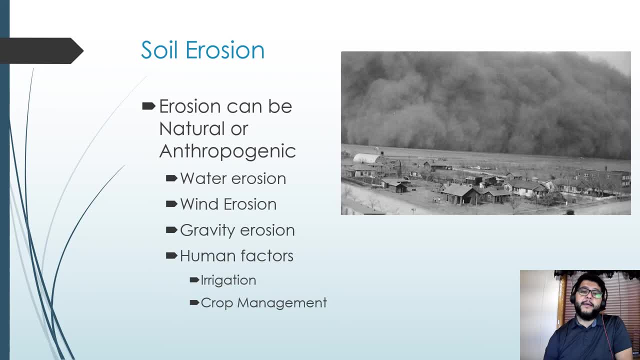 that it's caused by humans. okay, Human factors. So if you're thinking about how that can happen, that could be through water, wind or gravity, And then human factors can be through irrigation and crop management. So we didn't do very much of that around the Dust Bowl, And so you had these.